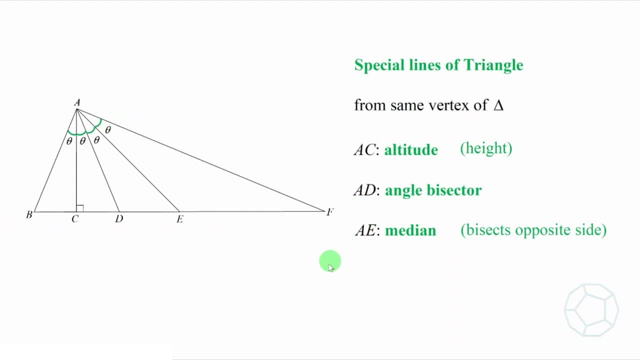 to find angle BAF We should make use of the powerful angle bisector theorem. So what's the theorem about In triangle ABD? C is a point on BD, so that AC is the angle bisector of the angle at A, Then the ratio of the blue size AB over AD. 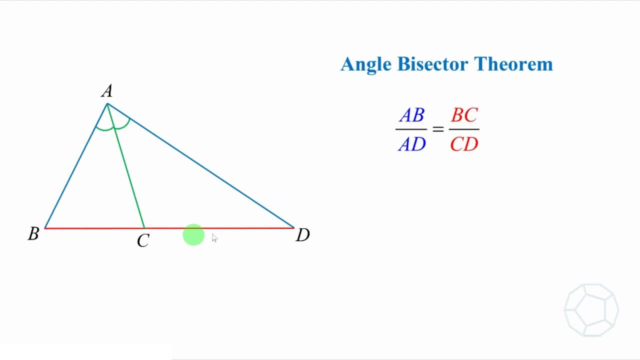 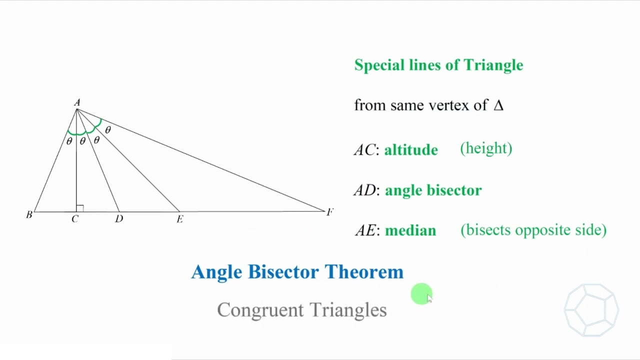 is equal to the ratio of the red size BC over CD. This theorem is proved by three different methods in another video. If you are interested, you may want to check out the link in the description. Great, everything is ready. Let's start looking at two congruent triangles. Can you figure them out? 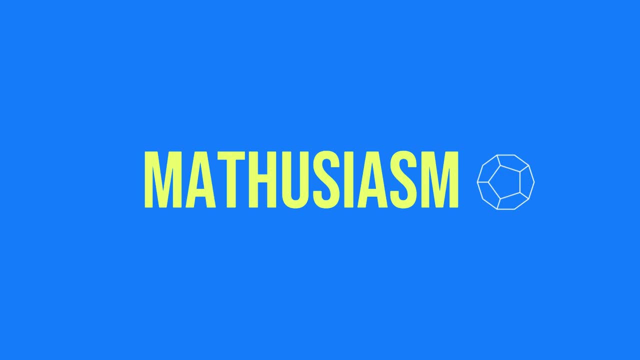 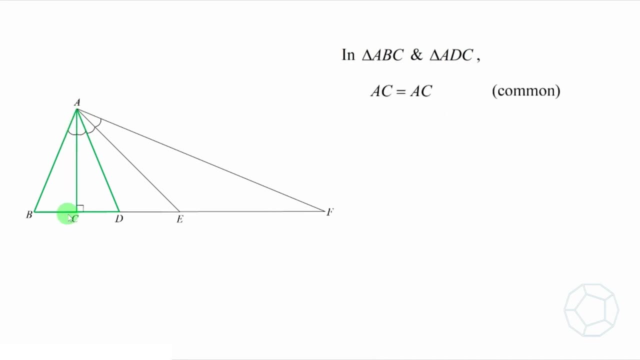 Let's focus on triangle ABC and triangle ADC. First of all, the altitude AC is the common side of the two triangles. Moreover, the two angles, C1 and C2, are 90 degrees. Also, A1 and A2 are equal. 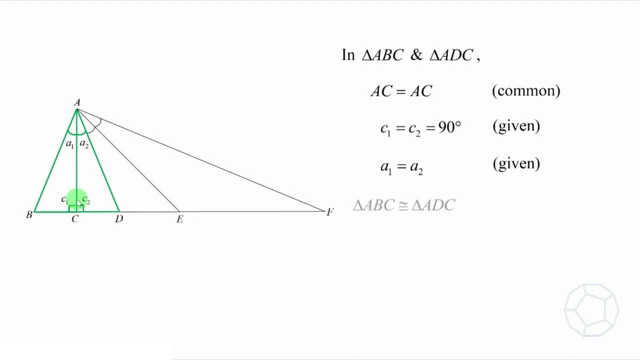 It's given at the beginning. Therefore, the two triangles are congruent and the reason is ASA. Now we have two pairs of corresponding sides of congruent triangles. Then we have: AB is equal to add and BC is equal to DC. applying the link of A to AB, 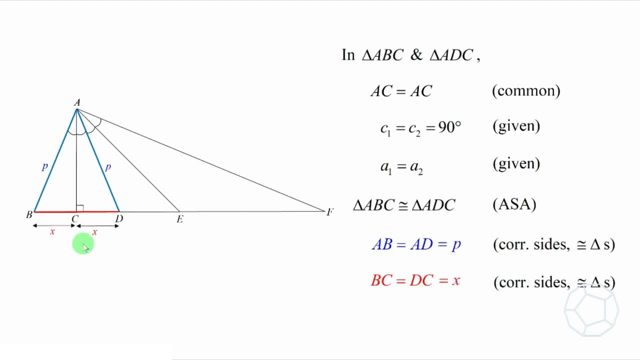 Denote the links by P and X respectively. For the sides from point A, we color them in blue. Let AC is equal to Q, AE is equal to R, AF is equal to S. Then we color the horizontal side in red. 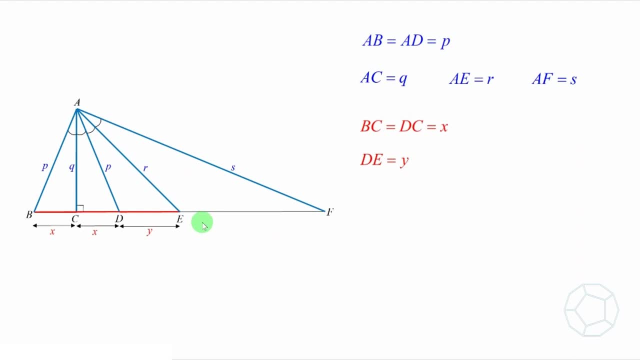 Let DE be Y length of EF, Because AE is a median of large triangle. therefore, EF is equal to BE, which is the sum of the three parts. therefore is equal to 2x plus y. Alright, we can apply the angle bisector theorem. Bear in mind that the ratio of blue size is 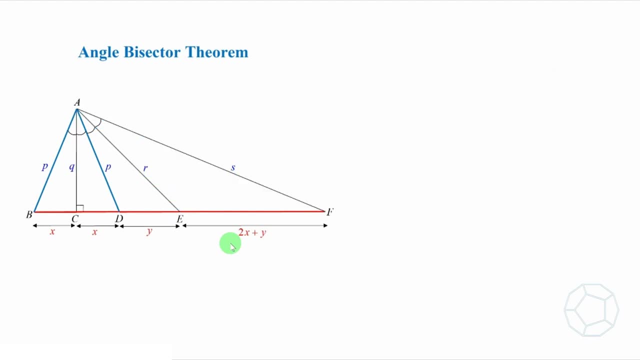 equal to the ratio of the red size. Let's choose two triangles with some equal size. The calculation will be much simpler Here. AB is equal to AD equals to P. Take the side AF as well. We shall consider triangle ADF and triangle ABF In the following the angle. 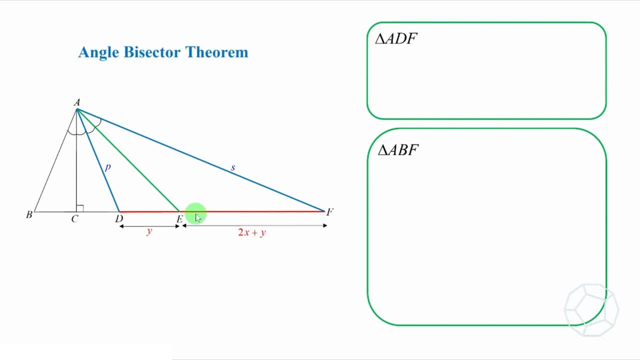 bisector is in green. for easy reference: In triangle ADF, AE is an angle bisector. therefore P over S is equal to y over 2x plus y. Let's call this equation 1.. In triangle ABF, AD is an angle bisector. Here DF is equal to y plus bracket 2x plus. 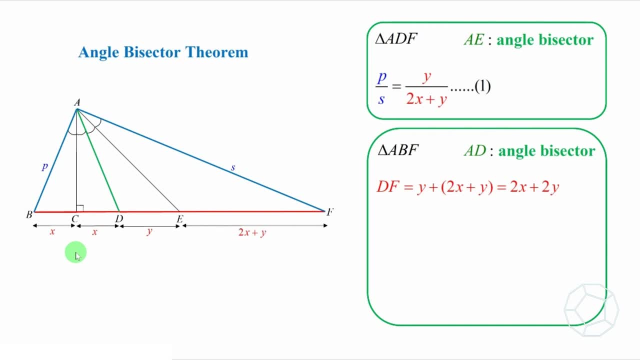 y, which is 2x plus 2y, And BD is simply x plus x, which is 2x. Therefore, P over S is equal to 2x over 2x plus 2y. Cancel out the factor 2 in the numerator and the denominator. 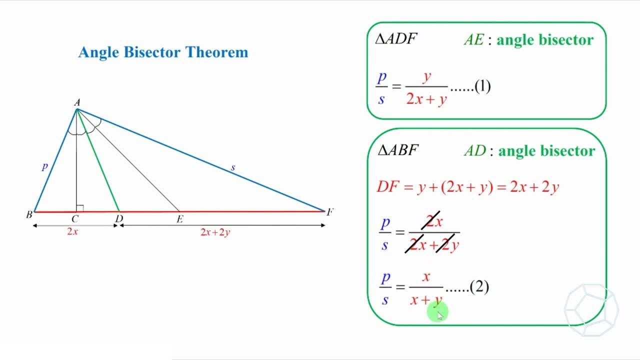 we'll have: P over S is equal to 2x plus 2y. Let's call this equation 1.. In triangle ABF, AD is an angle bisector. Here, DF is equal to x over x plus y. Let's call this equation 2.. 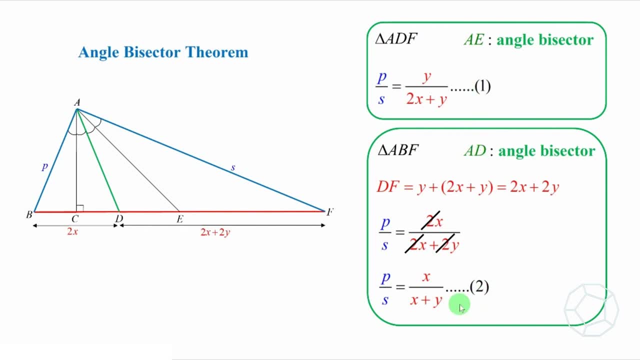 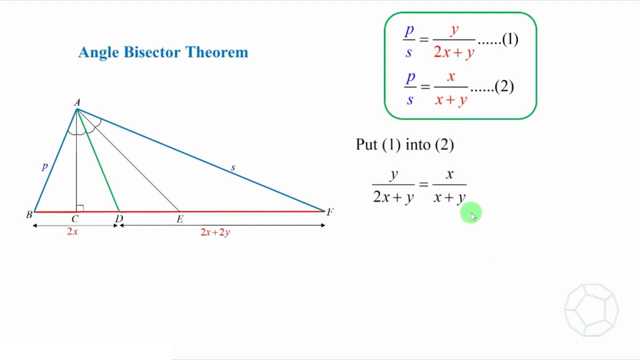 There are so many unknown lengths. What can we do Now? putting equation 1 into equation 2, then we get this Cross multiply to get rid of the fraction. it becomes xy plus y square is equal to 2x square plus xy. 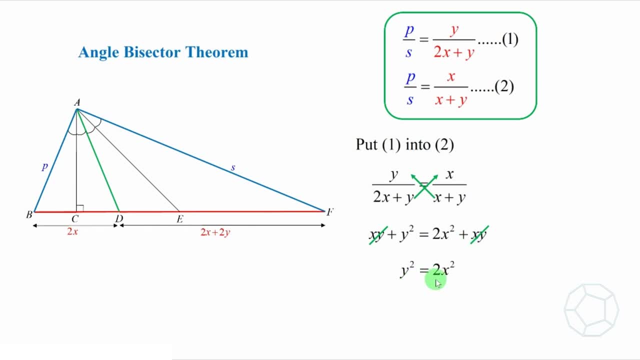 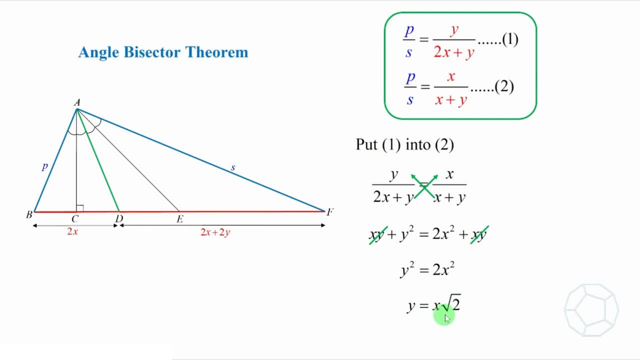 Cancel out xy on both sides, then y square is equal to 2x square. Taking square roots, we'll have: y is equal to x times square root 2, or negative x times square root 2, which is rejected. We have a really important relation between 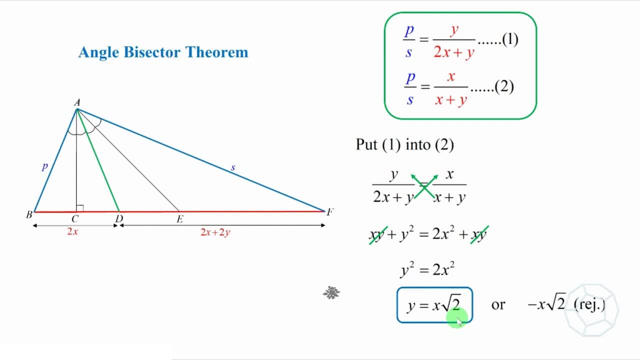 the sides. but what about the angles? Let's look at triangle ACE where AD is the angle bisector. By the theorem again we get: Q over R is equal to x over y. Let's put: y equals to x times square root 2.. 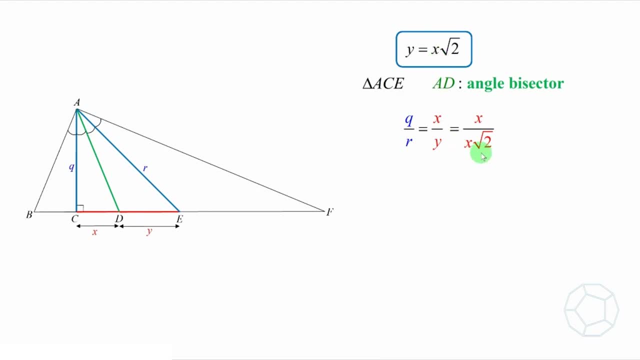 Cancel out xy on both sides, then y square is equal to 2x, square 2 into the equation. Then cancel out the x terms. therefore q over r is equal to 1 over square root 2.. Still, it's about the lengths. However, let's look at the figure carefully.